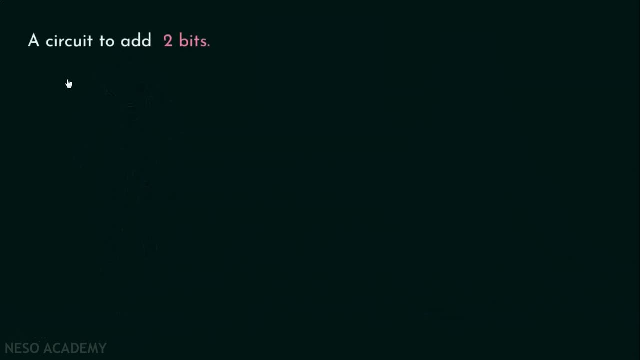 the final product. For an instance, if we are to build a circuit which can add two bits and produce sum as well as carry- I mean when both the inputs are zeros- the sum and the carry will be zeros Again, with two inputs and having one of the inputs as one there. 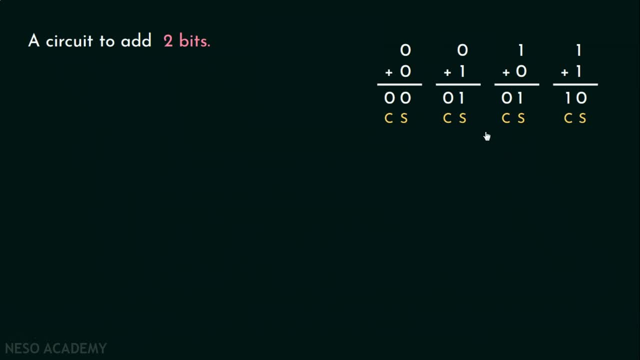 can only be two cases, And in both the cases the sum is one and the carry is zero. So if both the inputs are ones, the result is two. But since we don't have the symbol two in binary, rather it is represented as one zero. So the sum is zero and the carry is. 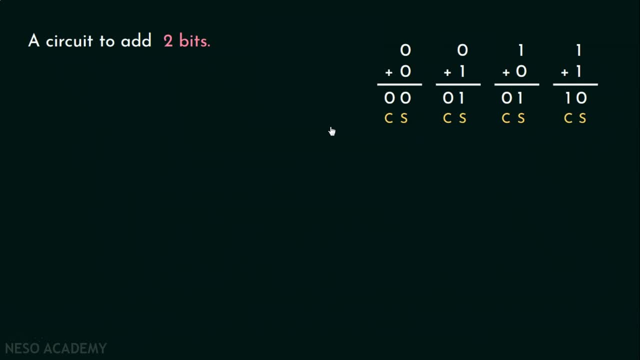 one. Anyway, we need not worry about the details right now because interesting discussions are awaiting. So in order to devise such a machine, first we need to determine the structure, then organizing the available resources, supposedly the universal NAND gates in this specific scenario. 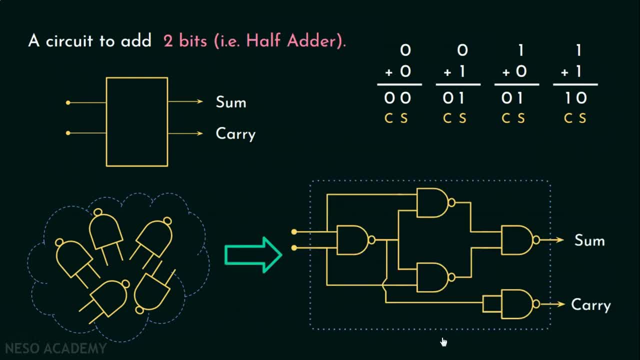 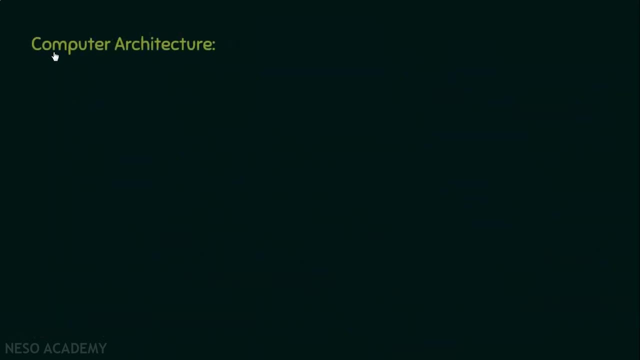 So we can build the half header circuit, which is nothing but the machine we intended to build to solve our two bit addition problem, Which means architecture and organization are systematic approach of deriving the solution of any problem. Now let's move on to the technicalities. So computer architecture basically deals: 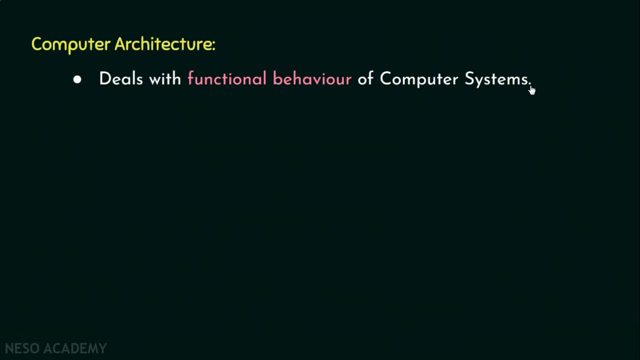 with the functional behavior of computer systems, And it is also all about the design implementation for various parts of computer. Now, coming to computer organization, it deals with structural relationship. Basically, the functional units collectively work together in order to execute computer instructions, So operational attributes are linked together. 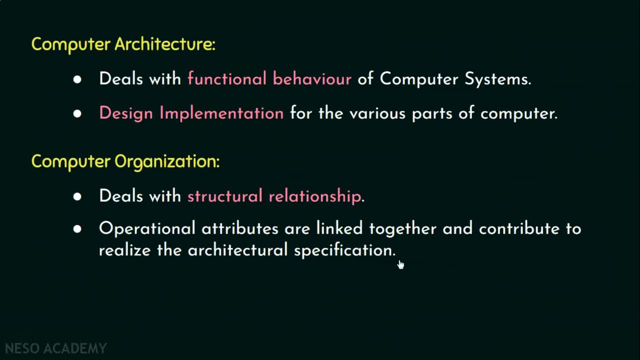 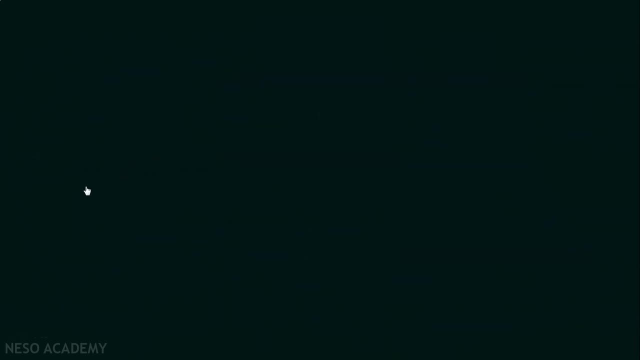 and contribute to realize the architectural specification. So, to sum it up, the designing is the attribute of computer architecture, whereas utilization happens to be the attribute of organization. Now, a generic computer is comprised of various functional units, Amongst them the processor. 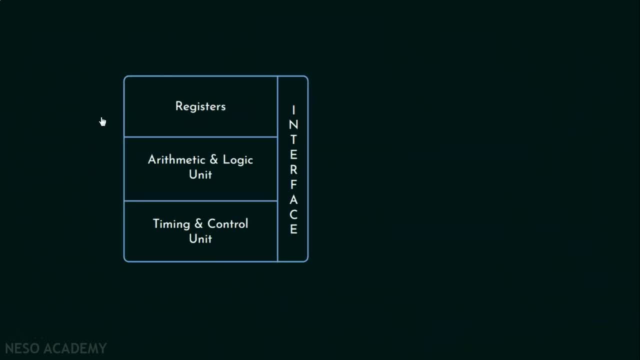 is the most important. The processor itself is a collection of register section, an arithmetic and logic unit, also known as ALU, and a timing and control unit. Along with these, it also has another section called interface. We can think of the processor as the brain of the system. 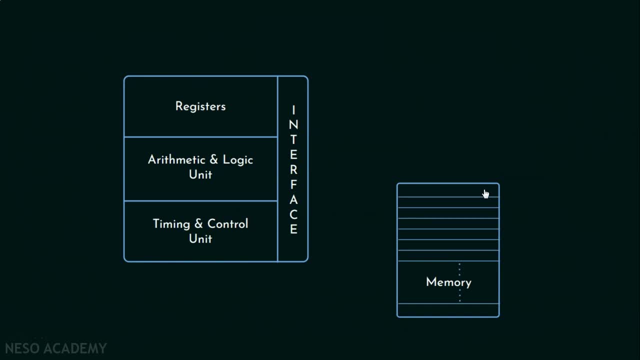 Next we have the memory. It stores all the instructions, reading ways. the processor works accordingly. Also, we can store data inside the memory. Another functional unit is the input-output peripheral. Now the term peripheral is just a fancy version of device. All of these are very essential. 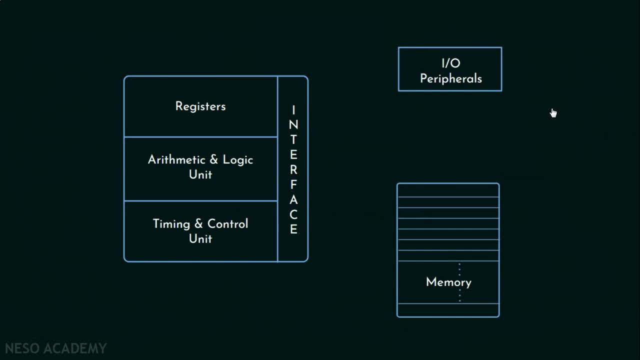 when computation involving computers are concerned. So the programs or the set of instructions are stored into the memory using input devices so that the processor can execute them. During execution, the required inputs can either be fed into the system using the same input peripherals or stored into the memory beforehand. Finally, the outputs can be generated onto. 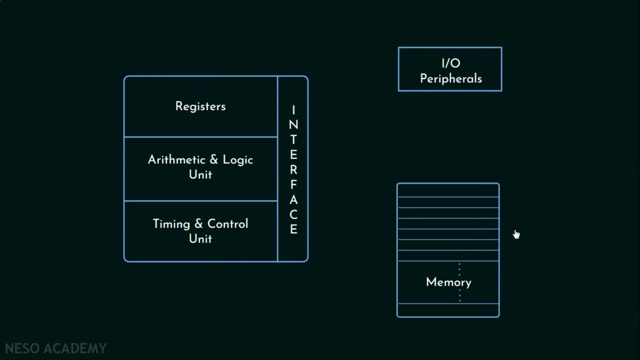 the output devices, Or else can be stored into the memory for later extraction. The intercommunication of all these functional components is carried out with the help of system bus. We will get to know about all these in a much more elaborated manner in. 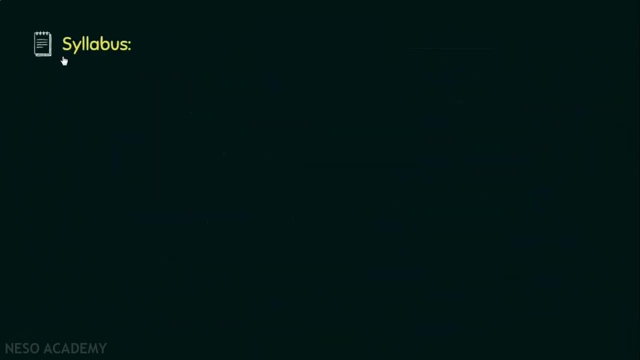 our due course. Now, coming to the outline of the course, that is, the syllabus that we are going to follow is as follows. First we will begin with the basics of computer architecture. Also, we will learn about the various classifications of it. Next, we will learn about memory interfacing. 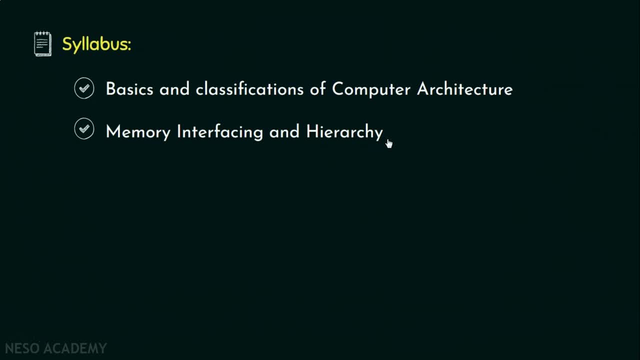 and hierarchy. Now in this particular section we are going to learn how the memory devices are connected to the processor, also the way the intercommunication takes place, And by the end of this we will have a pretty detailed knowledge of all sorts of memory mapping techniques. 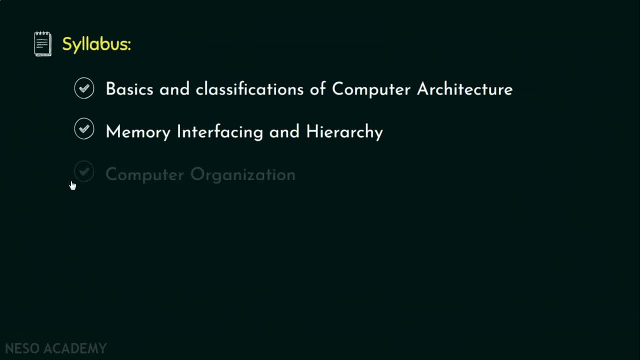 and a decent idea about the secondary memory storages. Now comes the big part, the computer organization, Starting from machine instructions, addressing modes, then the detailed organization of ALG, the data path and finally different types of control units. All of these we will learn in an eventual video. 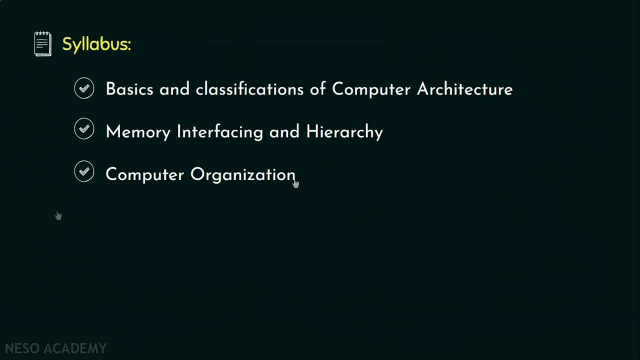 Thank you for watching. Next up is I-O interfacing. Here we are going to be introduced with the ways I-O peripherals can be interfaced with the processor. Also we will learn about various data transmission modes. Then we will learn about the instruction pipelining, which is sort of optimization. 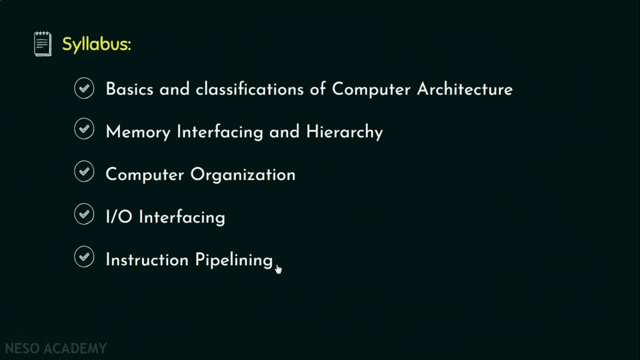 Basically, we will see how to increase the efficiency of a single processor And finally, a bonus section: number systems. Now many of us may argue that it is a very basic thing and very commonly known. We are learning it because this specific section has specially been designed keeping